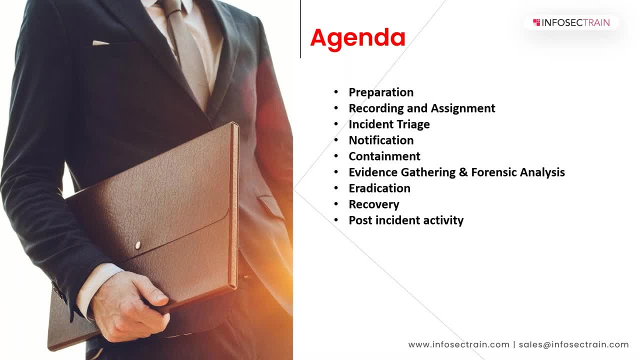 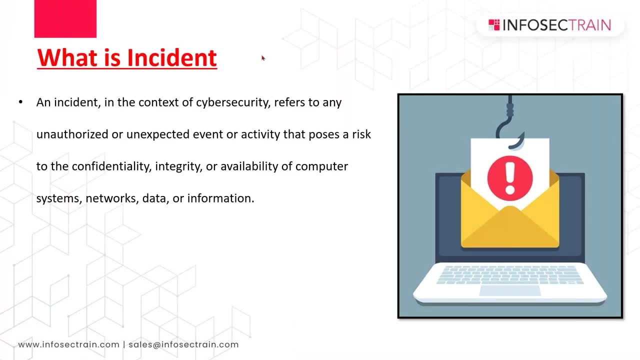 we jump into that and talk about this. the very first thing is: what do you understand by the term incident? What is incident for you guys? So event is, like we can say, occurrence of something or any activities which is being done right. So I used to give this example. 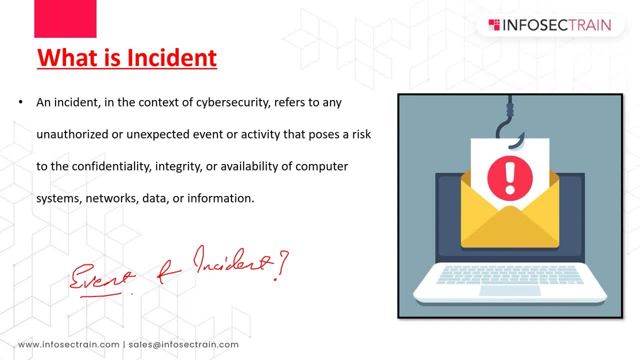 a simple one, Like: if I drop a bottle of water, that's an event. right, If I drop a bottle of water, that's an event. But if I say I dropped a bottle of water and it fell on my foot, I got an injury out of it, then it will be called as your incident Makes. 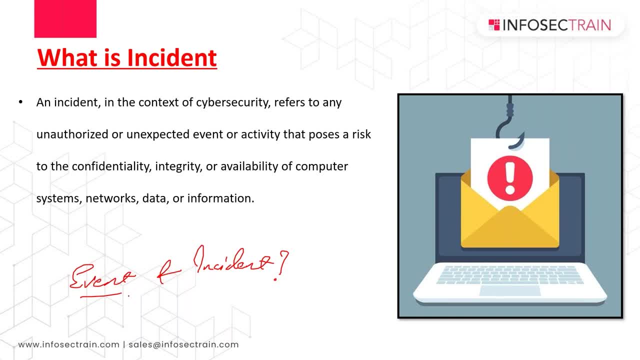 sense. So you know you plugged out your charger from the wall socket event. but somehow, if it corrupted it, it will not get connected. So you have to figure out what happened. your system incident right, you plugged out your- you can say you know- hard drive from a laptop. 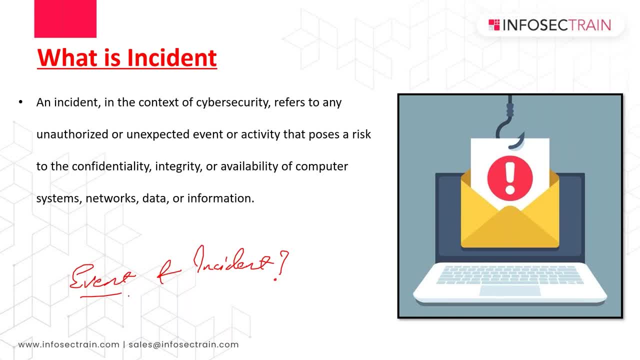 without having a proper you know, ejecting it, so even, but it corrupted the entire data of your hard drive incident. right, so every incident can be an event, but every event cannot be an incident. okay, so an incident when we're talking about uh, in the context, cyber security refers to any. 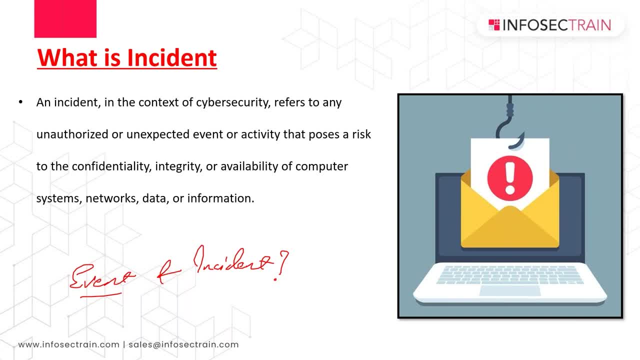 unauthorized or unexpected event or activity that poses a risk to the confidentiality, integrity and availability of computer systems, network data or information. right confidentiality, integrating availability, confidentiality, as in another, like you know, swapping from any, any unauthorized access. integrity verifies that your data is accurate. it is not tempered, it hasn't not been. 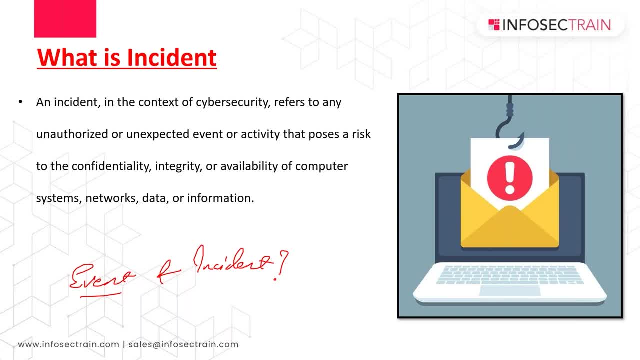 modulated, and so be it. these are the two. then the second point: okay, that's the right. gewa returns- it is, like you know, the same, the original one. availability: your data and services are available to its genuine users here. so, basically, your incident typically involves a security breach. 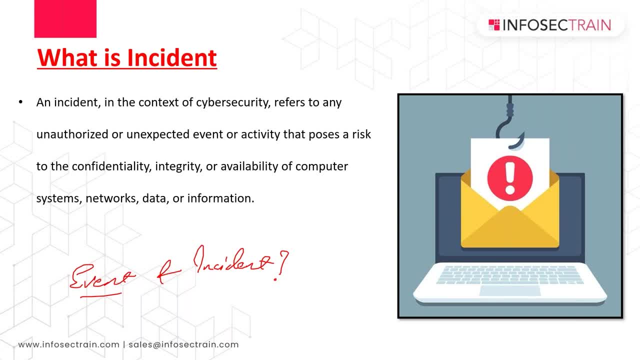 violation or compromise that may result in damage or any kind of a loss or any kind of a disruption to an organization's assets or their operations, or repetition as well. okay, so see like, while it's not possible to completely animate, uh, or possible to completely eliminate the risk of incident, you can take proactive measures to reduce the likelihood and impact. 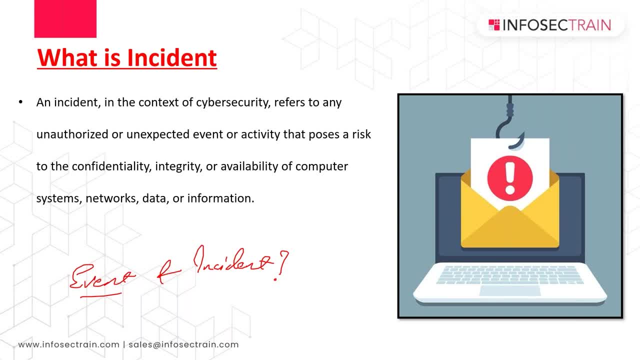 of security incidents. okay, proactive, as in two things are there right: proactive and reactive. proactive are something, something which are you taking before and in order to prevent yourself. reactive is something has happened, then what you are doing correct, so this is incident. so, for the same thing, when we talk about incident handling, so incident handling is effective. 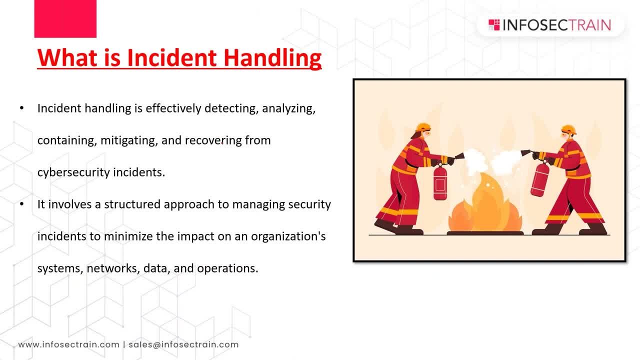 detecting, analyzing, containing, mitigating and recovering from cyber security incidents. so it involves a structured approach to managing security incidents to minimize the impact on an organization's system, networks, data and operations. okay, basically we have actually steps in place to handle and respond the incident in an organization. 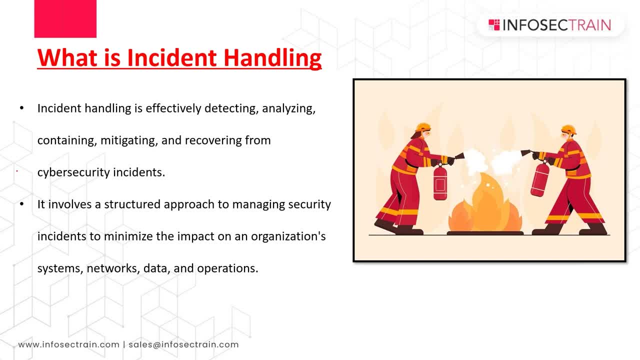 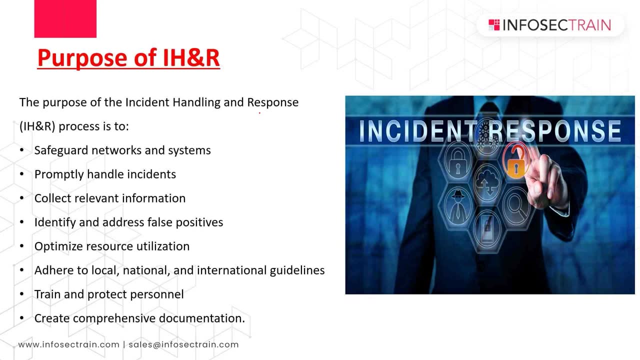 which is implemented properly, uh, it will cut down or reduce the impact of the incident on the organization. okay, so incident handling and response when we talk about, there's a purpose of it. the purpose of instant handling and response process is to networks and system promptly handle incidents, collect relevant information, identify and address. 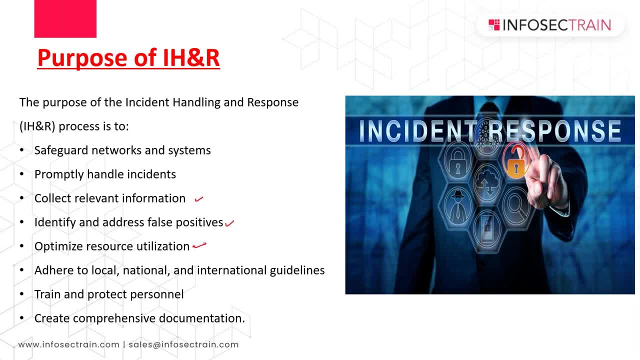 false, positive. optimize resource utilization. adhere to local, national, international guidelines, as in getting compliant, right, okay and following the proper standards, right, train and protect personnel. create comprehensive documentation like it's like documentation are done so that you can, you know, learn about your organization so that you can improvise a security posture. more so once. 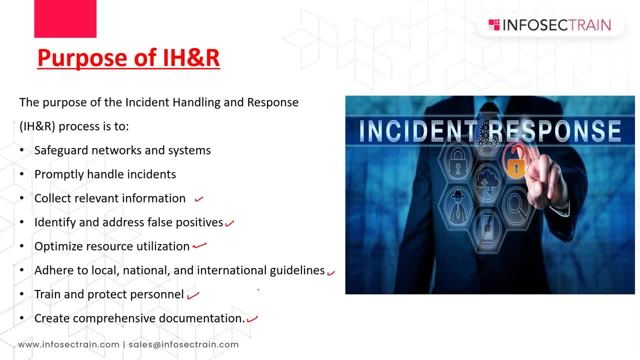 an incident has happened. you know you you mitigated it, you handle that incident properly. you know you took certain steps. so later our documentation will also be done and you'll find out, like you know what, whatever weak point, why we got attacked. you know how the attack happened and what we were. 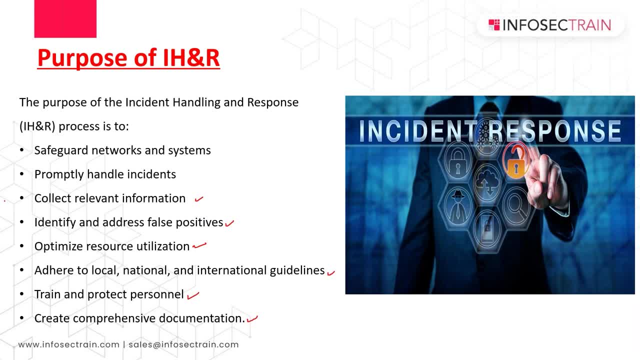 lacking. how can we more stronger if new controls are required implemented? you know those things. so, basically, documentation helps you to create, increase or make your security posture more and more better of the organization. okay, here, one thing is use: identify an address, false positive guys, what is false positive? so it's like our alert. two things are there, guys, in terms of this alert. 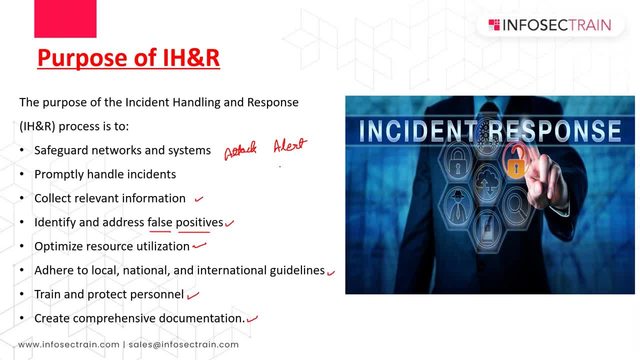 and attack is there okay? so if you're getting a notification and alert from us, you can say this. and for fact, there are three safety controls: alert safe and not bathroom or detects, not safe. do you want to do um forô you react? you'll do what has to be honest, but you have to be completely honest because alert is an wykor捅it. yJeb's REALTIME is NOT called A LIE CON. 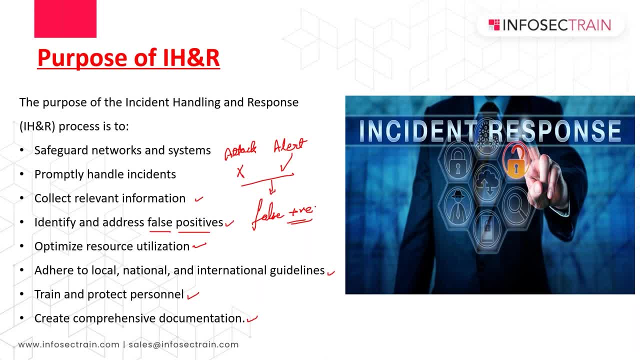 for the rules conditions were met. so alert generator like alert was generated and tells that, okay, there's an attack going on, but in reality there was no attack. so simply you can say: let's suppose if deepak is there, for example, deepak is trying to log into his account, right? 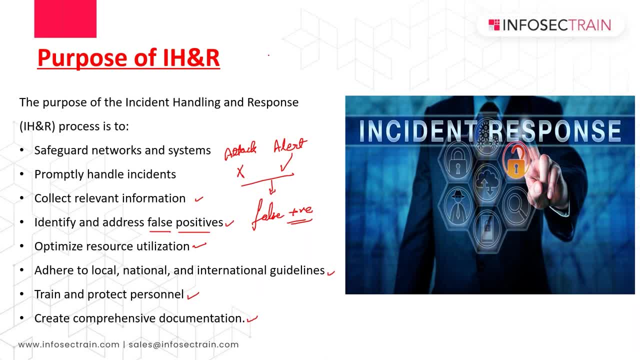 and like there was a rule. for example, there was a rule that if there are failure attempts, login failure attempts which is more than three for the same account and within five minutes of a time frame- okay, within five minutes of a time frame, so raise an alert if such conditions is met. so if we say that, let's suppose deepak is there and 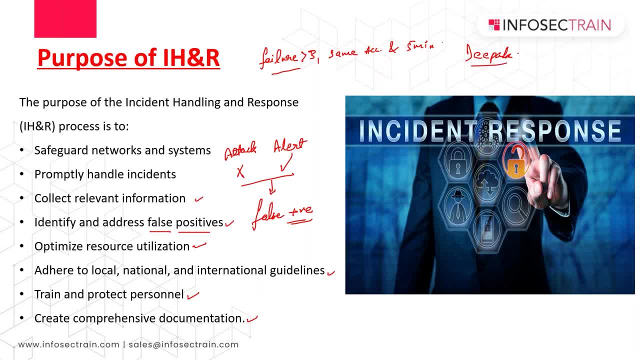 deepak is an employer. okay, he's an employee of an organization. so he was trying to log into his account and he made four failure attempts. four failure attempts. so, as per this condition, four failure attempts within five minutes. as per this condition, it will raise an alarm. right, it will raise an alert that someone is trying to. 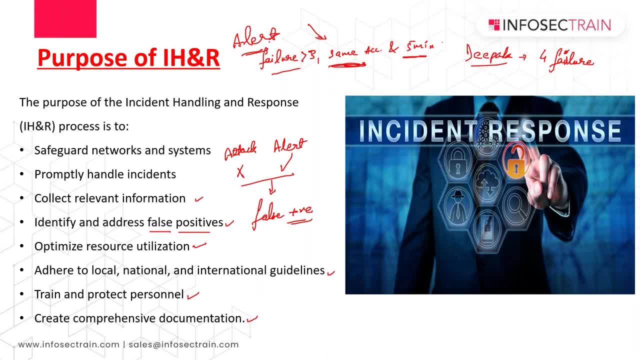 attack or guess the password or crack the password correct. but when we cross checked, in reality it was deepak only. it was a genuine mistake which was being done from deepak's end because he's an employee. okay, he forgot his password, so he was just trying to enter multiple times. so then it becomes your. 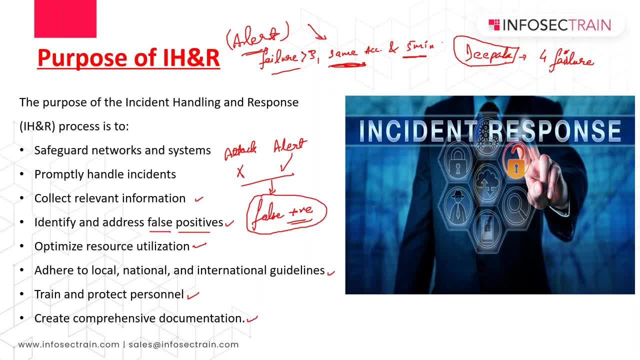 false positive because what it was? not an attack, it was deepak, only he was accessing his account. makes sense, rajesh, it will be considered okay. true negative: jp2: we'll talk about later. if you have this query, we can discuss. i can explain all those things later, okay, because it will be time. 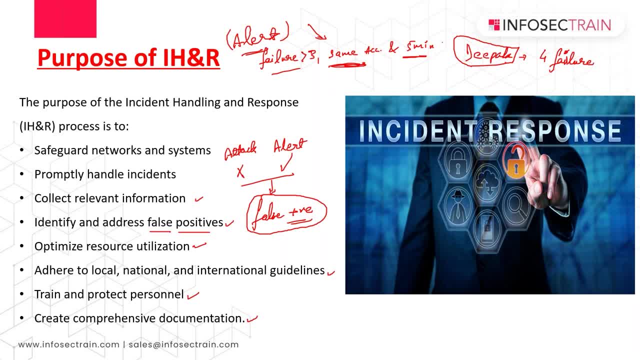 consuming us for now and it could be considered insider threat as well. but yeah, as i mentioned, this will be checked right, rajesh. and inside of that, he see he already have his access right. he already know about his account password, so we cannot say insider threat because deepak is actually trying to enter his into his own account. 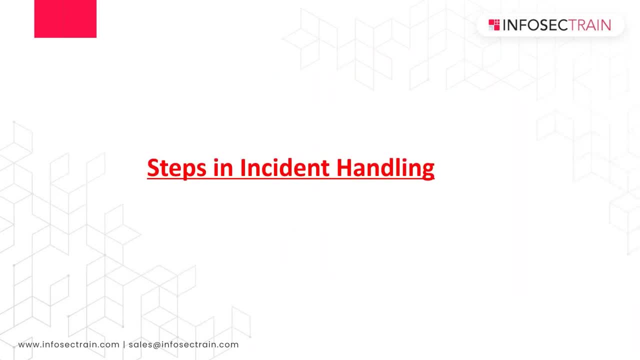 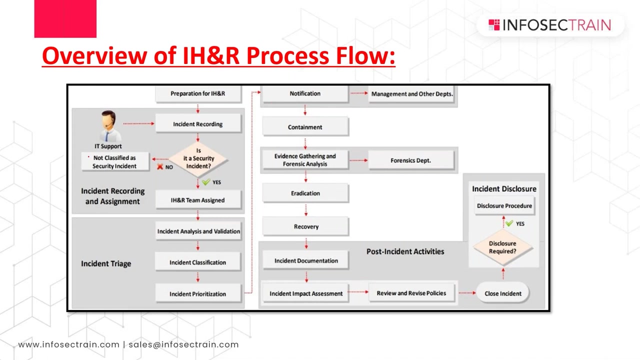 next thing is steps in incident handling, which you are discussing in the starting right. so i have what i have- uh, given this images, also a pretty good, you can say, overview about this entire process of instant handling, like what happens at what particular time and all those things are mentioned over here. okay, so here you go. um, we have preparation for instant. 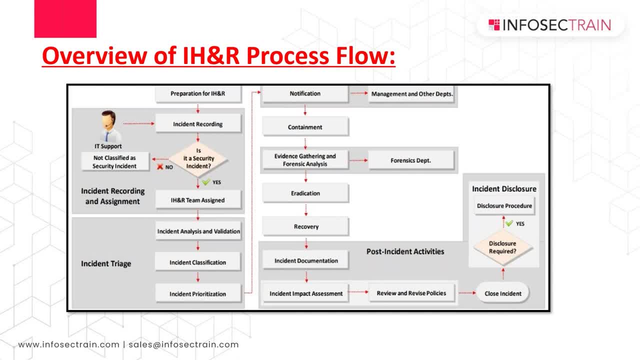 handling and response. we have uh, instant recording, an assignment in which these things are there. instant triage is there. then we have notification containment, uh, evidence gathering and forensic analysis, eradication, recovery and post-incident activities. basically, this is the entire flow of how things are. you know, whenever an incident happens, how it goes through through these certain 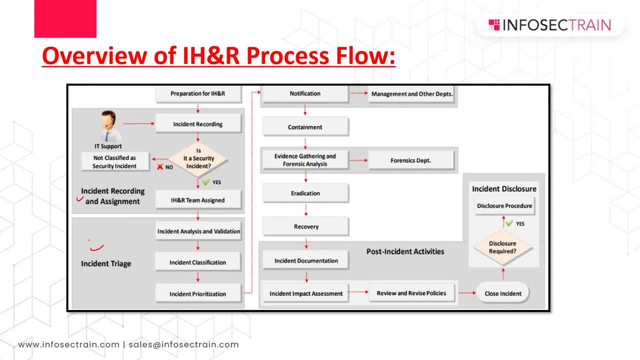 steps or phases. so this is the key thing which i mentioned over here for you guys. okay. so very first one is all preparation, then it goes to instant recording an assignment like, then it goes for instant triage where classification, verification, prioritizations are done, then it goes. 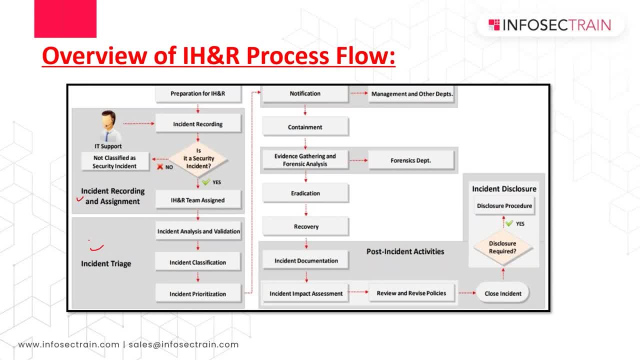 to your uh notification. notification, as in, it's being notified to your stakeholders, to your management, and then approval is also taken and meanwhile you can see the containment is done. containment is, uh, it's like an isolation. okay: evidence gathering, forensic analysis and then eradication, recovery and post-incident activities are also there. so let's get into each step one by one. 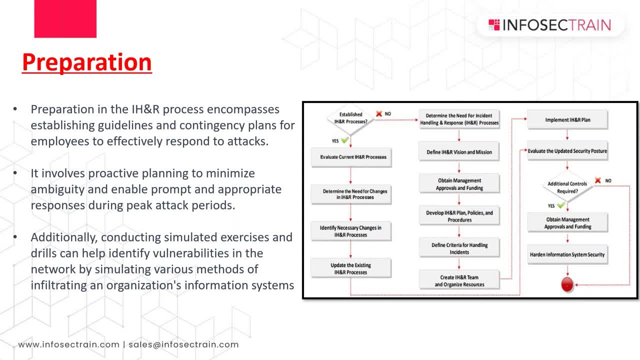 perfect so preparation and incident handling response process. it can encompasses establishing guidelines and contingency plans for employees to effectively respond to attacks. it involves proactive planning- right, proactive before, and we are trying to uh fix up things over here so that you know we'll try to um align everything in place so that in case if an attack happened, 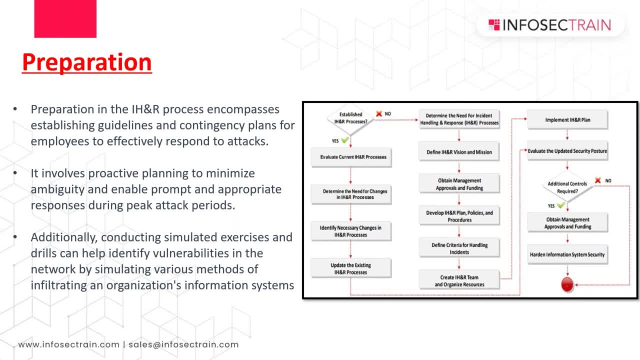 first, we will try to make sure that it doesn't happen at all. but in case it happens, how to proceed ahead with that right, how to quickly respond to that? that's the point: proactive approaches. so it involves proactive planning to minimize uh ambiguity and enable prompt and appropriate responses during peak attack periods. uh additionally conducting 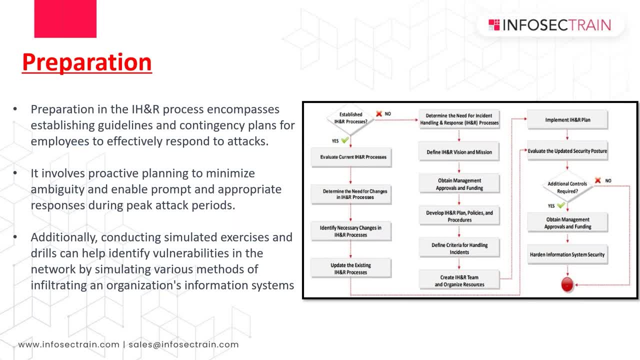 simulated exercises and drills which can help identify vulnerabilities in the network by simulating various methods of infiltrating an organization information system. right, the simulator exercise will be there so that we can check whether we are having any vulnerability or weaknesses present on ourselves or on our network or not, on the very first place. right, so as just. 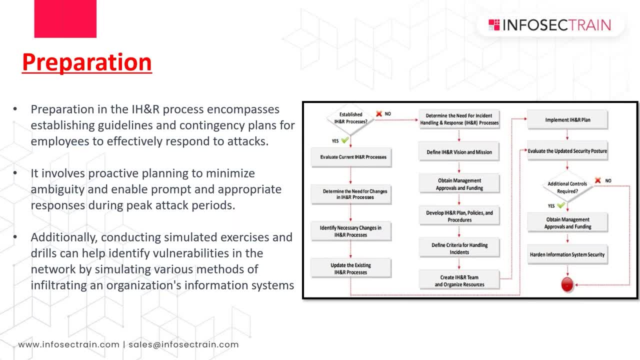 mentioned. in this stage, you can see, the organization will define the mission, vision and scope of your instant handling and response. okay, they will also obtain the management approval and their funding. they'll be developing and, you know, implementing security policies, building an instant response team over here, right, uh, gathering systems, hardwares and software tools which are 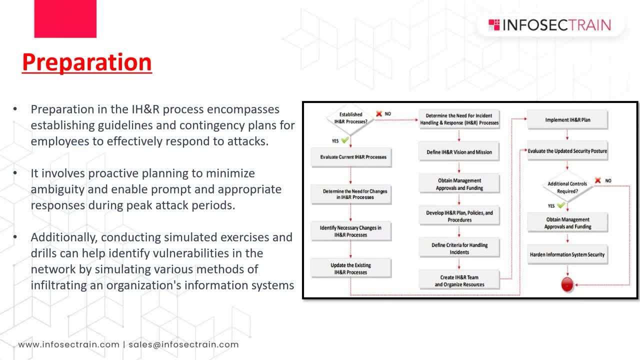 required, for instance, response. we are prioritizing the assets over here and the services. we'll create a plan for smooth communication whenever an incident happens, because a communication is also required, so that whenever- because it's kind of a panic situation, so smooth, you know- communication should also be there already. 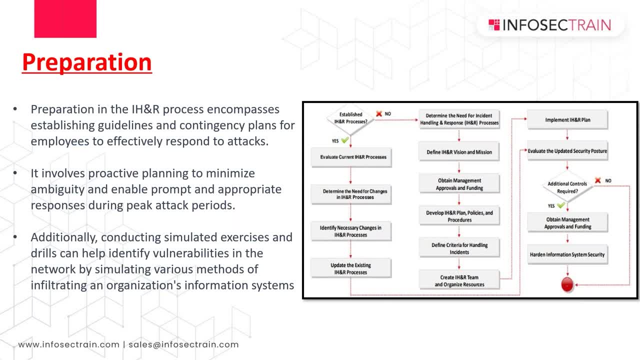 prepared. so preparation is all about that. okay, so we check whether you have any uh established, already established. you can say incident handling and response process or not. okay, you already do. you have already like a process already into the organization placed or not. you check for that in the very first part. so it's not. 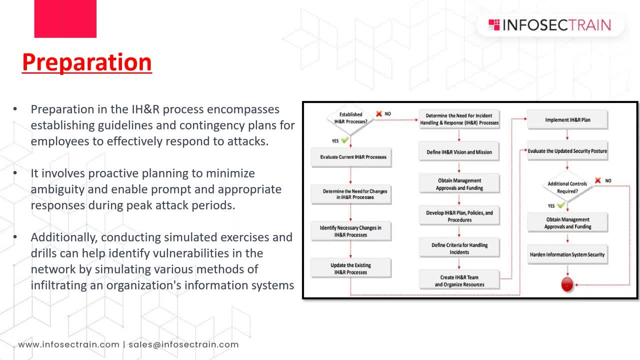 there. so if it's not there, then what you do? then you go for determine the need for incident handling and response process. okay, you determine the need for incident handling and response process. organization to determine the need for incident handling response process based on their current security scenario. their 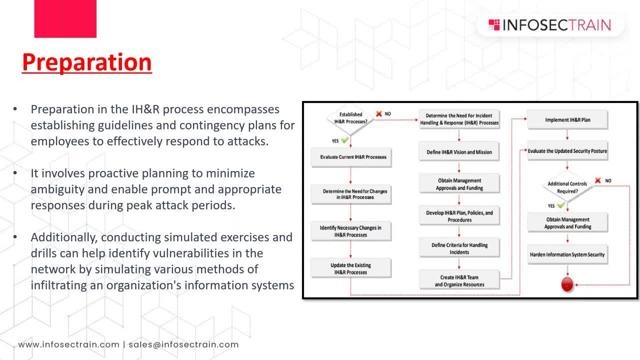 business advantages of having such processes, their legal compliance requirement, right organization policies, their previous incidents, on all that. okay, then they define their instant handling, response, vision and mission. okay, so this vision statement: basically, it will be reflecting your organization's middle, mid and long term goals for incident management capabilities. okay, so that will be a vision mission would be like. 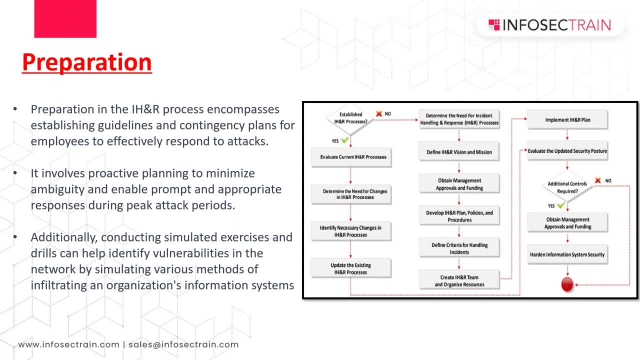 you know, uh mission statement will be defining the purpose and the scope of the planned incident handling response capabilities. okay, so define the vision and mission, then management approvals. obviously see, without funding can we do anything, guys. so instant handlers, they should obtain the proper permissions from the management, from your stakeholders and your other authorized uh personal. 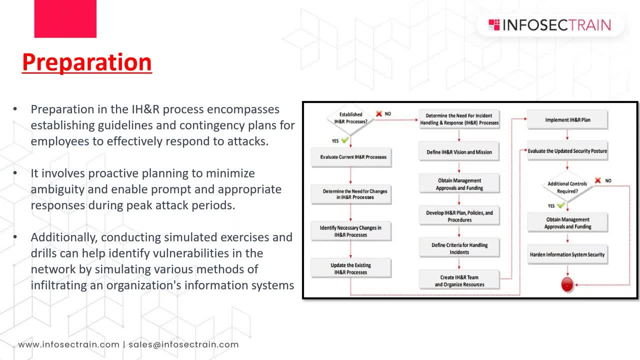 okay to execute your instant handling response process. so determine, like you know, funding requirements, uh, based on your assumptions of instant handling response capability components. so you justify basically fund requirements with your business analysis. okay, so that basically cost will include for various things no like for your team staffing. correct your toolkits. 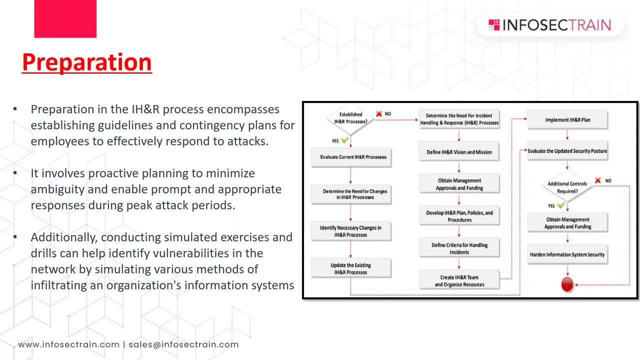 your communication systems for your space requirement, transportation, if third-party assistance is required. even for that, you know power, environmental controls, forensic investigations, so multiple things are there. so basically, obviously your funding will be required for the same right. then you develop an incident handling and response plan, policies and procedures, so basically a plan. 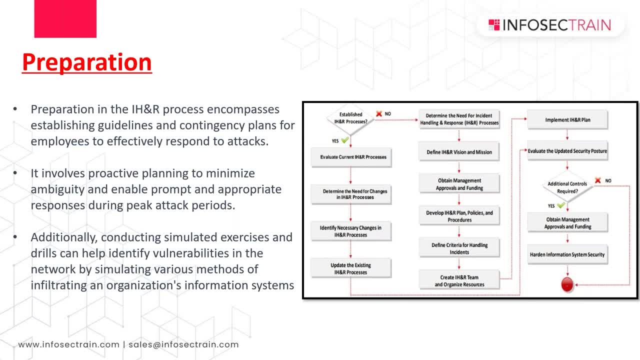 is there, which will be, uh, you know, determining the future course of actions, uh, for establishing, you know, and managing and strengthening incident response capabilities. so your incident handling response, it should, like, you know, it should include basically the address, the organization management statements and all that can be planned in order to easy to organize. done so. 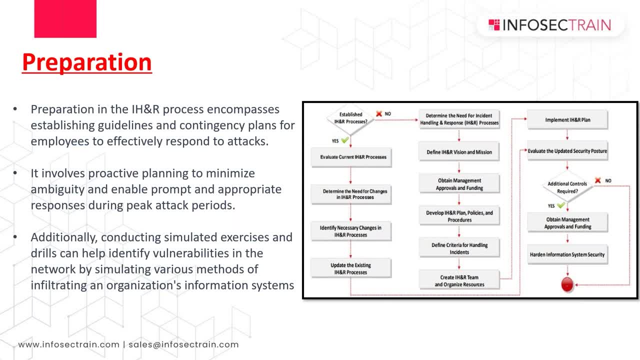 let's give another example real quick. we have w written a plan in the example, uh, the planning plan. it should include a plan areas you know like. checklist will be there tables, cheat sheet, flow charts that will be helping in decision making during your incident handling and response procedures. right, so you will also like 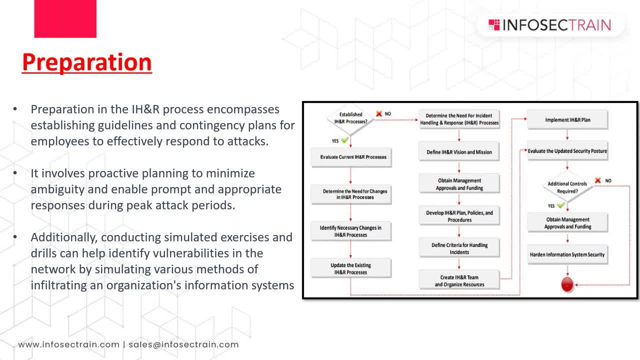 you know, you will create a checklist, you'll categorize what kind of incidents has already been happened, what kind of incidents are there. so this can like do the smooth process. so you'll define the procedures you know, so you develop the team, every organization they like, apart from. 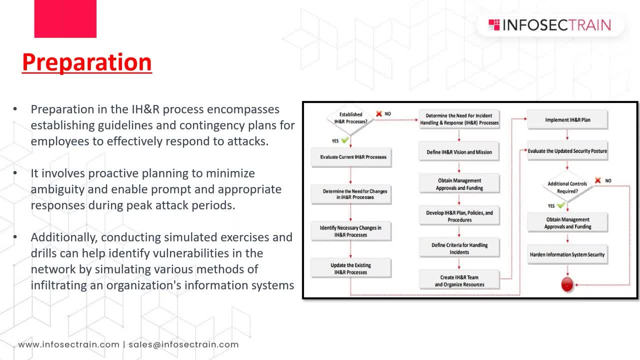 preparing the incident handling response team, your organization. they must define incident readiness procedures so in order to be, you know, equipped according with the necessary toolkits in order to fight with those incidents, right then, yeah, procedures will be there, criterias which were discussed and create incident handling response team and organize resources right. so this will. 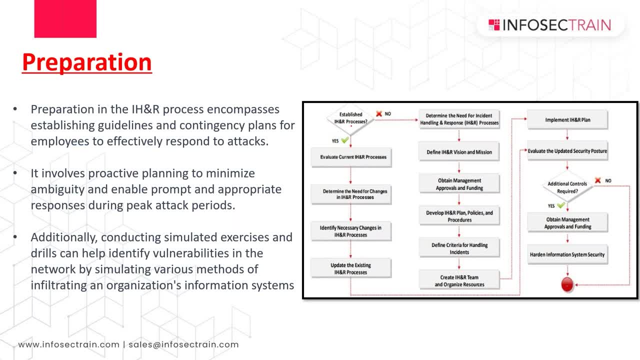 be when you do not have already a process established. if you do have, then you evaluate your current incident handling response processes, simply right. you determine the need for changes. if there is any changes required, you determine what are the need of changes for that particular process. you identify necessary changes in the incident. 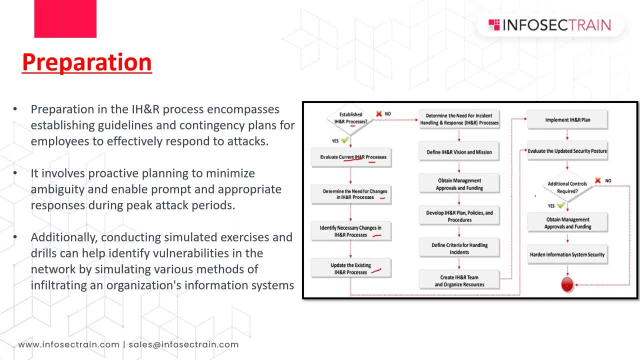 handling response process. you update the existing processes, then you evaluate- yeah, they both reach to the same point. right after plan, you will it updated security posture. okay then, additional security in order to, you know, increase the security posture. if not, anything ends over here. if yes, then again. 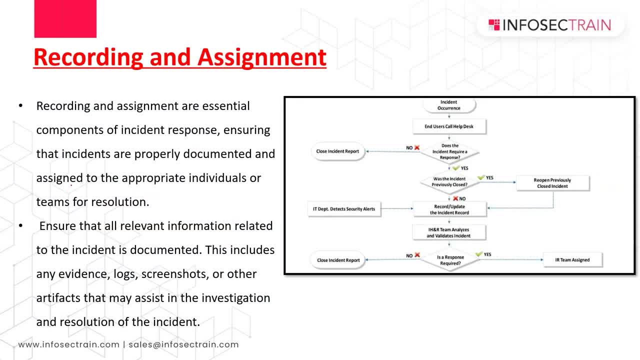 you obtain the management, approval and funding, then harden the information system security by that particular control. okay, so this is a process of your preparation, which is the very first phase of your incident handling and response process. then it goes to recording an assignment. that goes to recording an assignment. recording an assignment is there. basically, it is required to complete the equipment in order to use the water怕. 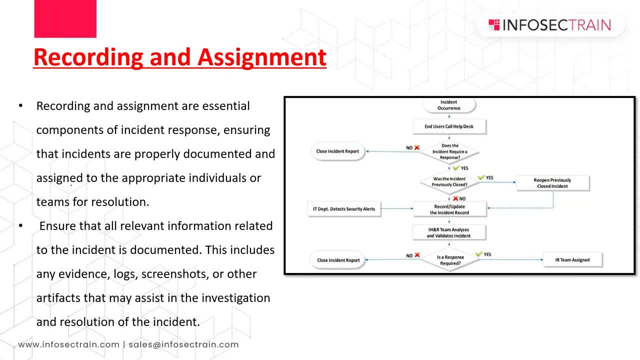 recording assignment. they're essential- you can say essential components of instant response. basically, ensure the nissans are properly documented and assigned to the appropriate individuals or teams for resolution. it ensure that all relevant information you know related to the incident is documented properly. it will be including all your, like you know, any kind of 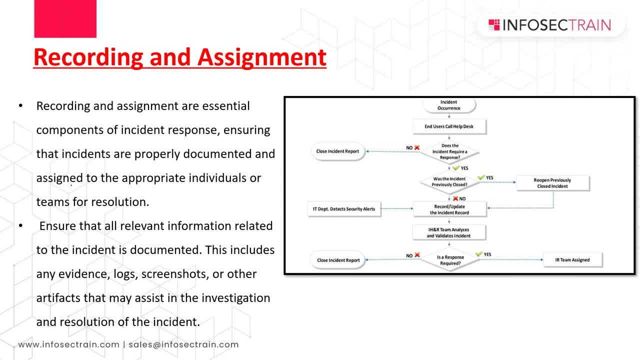 an evidence, logs, screenshots or any kind of an artifact that may assist in the investigation and the resolution of the incident. okay, so if an employee there finds any abnormal changes or indicators of an incident, then he or she they should immediately cross-check his or her database to confirm the changes and inform the help desk personally. so such as a system. 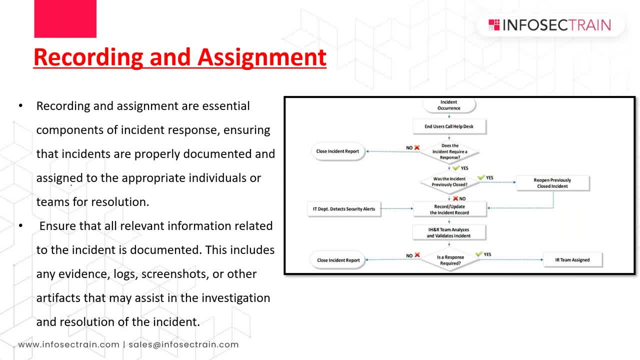 or network administrator about the particular situation. okay, so for our purposes you can say it is important to note here that a help desk consists of experienced instant handlers with years of experience. so help desk will accept such a request from an employee and conduct a- you can say- pre-eliminary. 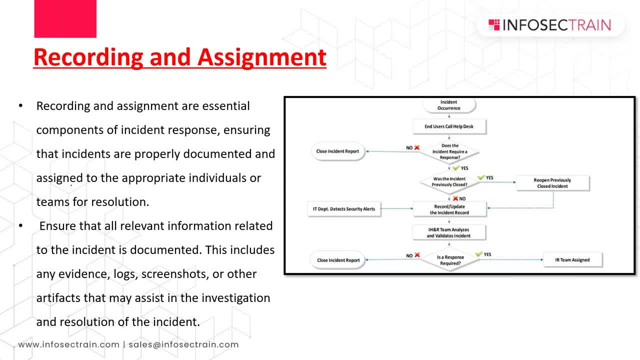 examination to determine whether the employee is reporting a valid intrusion or a breach from malicious sources. whether it's a valid or not, if the help text finds that incident did occur, then it will file a case for further inquiry. next it will try to determine whether the incident 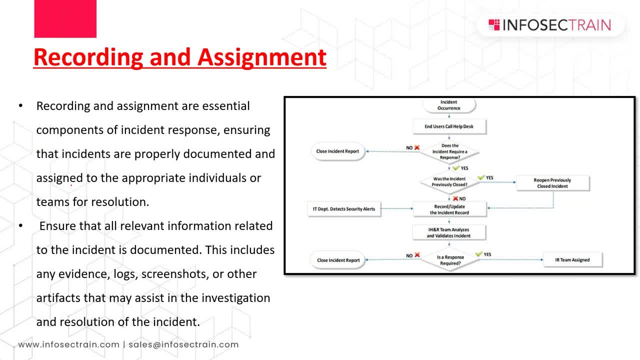 reflects any previous incidents and conduct further examination. so if the incident is found a mirror to any previous incident, then the help desk will reopen the previously closed incident and update the incident record over there. otherwise it will record it by collecting information about the incident, such as security alerts and the indicators from your id department. 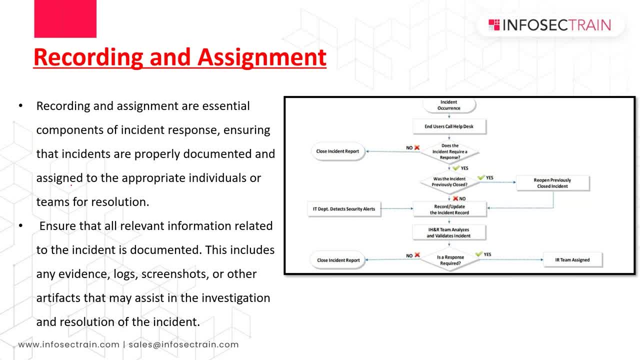 so this incident record is sent to the ir department incident response department for analysis and validation. so if the incident resource department or instant respond department finds the incident to be valid, then it will immediately assign the incident response team for further analysis. so we are just checking over here whether it is. 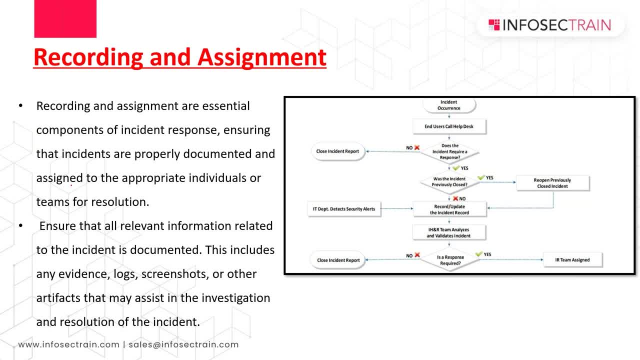 you know a valid incident or not. okay, so end user call the help desk. does the incident requires a response? no, then close the incident. if yes, was instant previously closed. yes, then we will reopen the previously closed incident and update the record if it was not previously closed record. 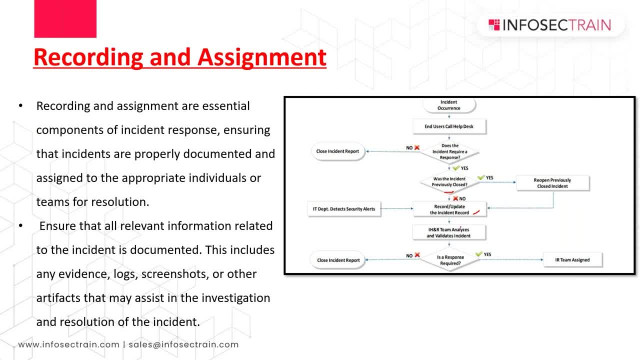 or update the instant record and then instead handling response team analyzes and validates the incident. is a response required, then team will be assigned to it. if it's not, then again we close the incident report right over there. then, after recording an assignment, that index phase is your instant triage actually. 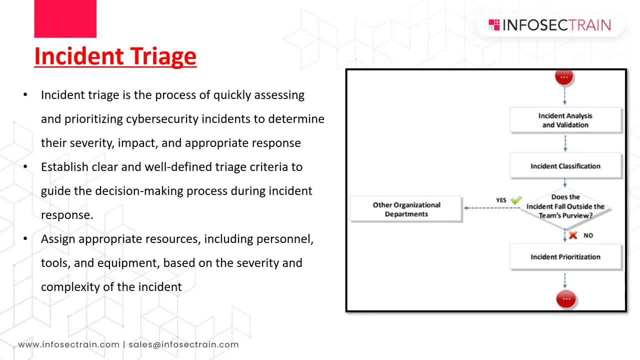 incident triage. your validation, classification and prioritization is done basically in part of this one instant triage. so instant triage is the process of quickly assessing and prioritizing cyber security incidents to determine their severity, their impact and appropriate responses. so they establish clear and well-defined triage criteria to guide the decision-making process. 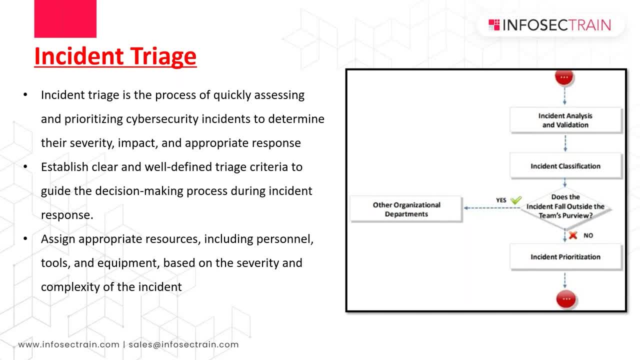 during incident response. so assign appropriate resources, including, like your personal tools, equipments based on the severity and complexity of the instrument. so, after incident, after incident recording and the same team assignment, your incident handling and response team is responsible for taking over and analyzing the incident with critical reasoning and good judgment. okay, so inside, 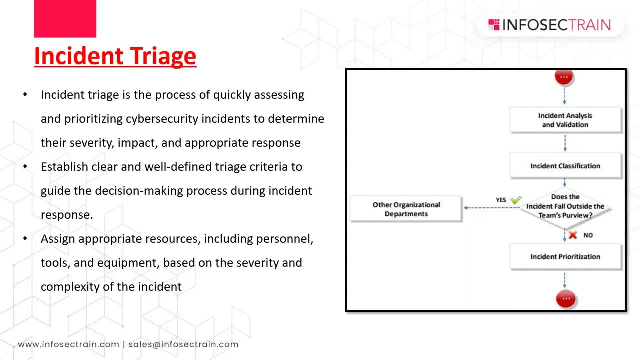 handling a response team. they should have a structured approach basically for, uh, efficiently report responding to an incident. okay, so along with this you can say incident handling a response team manager. they'll classify and they prioritize incident based on their- you know- risk level, whether it is high, medium or low. so teams should classify incidents and, you know, first attend to. 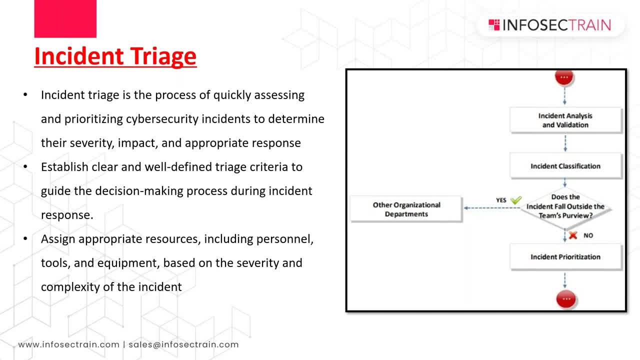 high priority incident, then medium priority incident and finally, and which is obviously the low level incident should be taken care of. okay, so after you can say you know previous step, you go for the instant. prior incident analysis and validation is done. okay, then instant classification is done, you classify the incident. does instant fall outside the team's purview? if yes, then other. 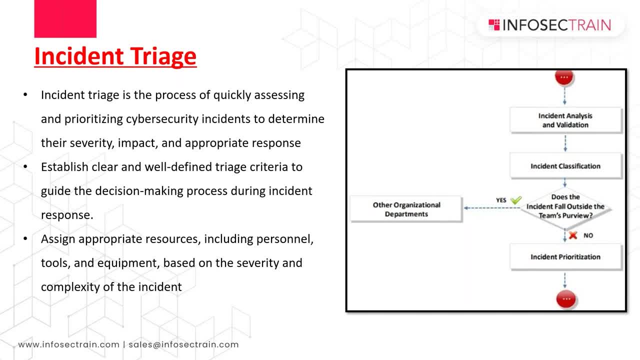 department will be handling it. if it's not, then instant prioritization will be done. you know, high, medium, low and as for that, the uh incident will be handled basically right. so instant triage and simple word that this will be involving, like you know, assessing your incident severity, its impact and its urgency. so, basically, 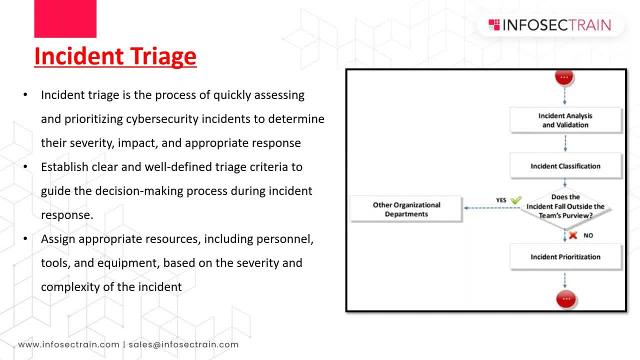 it helps to prioritize the incident based on their potential risk and determine the, you know, appropriate level of response and the resources which is needed. so simply, that's regarding that which is try it incident, try the third step and after this it goes for the notification. notification as in, as i mentioned, like you know, without management, approval, everything, anything. 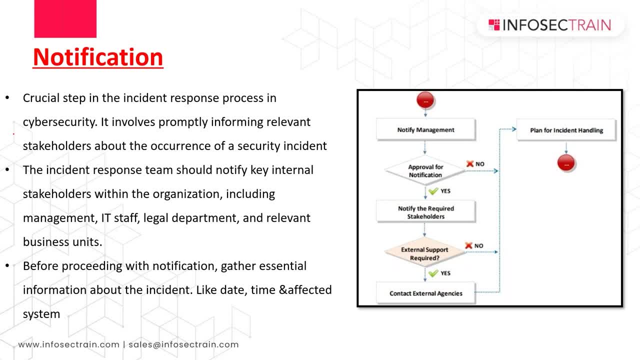 is not possible right. such thing happens in order to take further step, you have to have the approval right. so notification is like notifying your management, your stakeholders. so crucial step in the incident response process is in cyber security. it involves promptly informing relevant stakeholders about the occurrence of a security incident. the incident response team should notify key internal 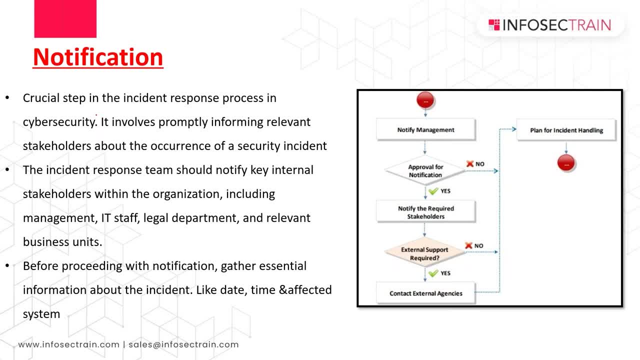 stakeholders within the organization, including management, IT staff, legal departments and relevant business units, before proceeding with notification, gather essential information about the incident, like date, time and on the system which has been affected by the particular incident. so you know, after completing the instant tries phase incident handling response team, they will be aware of the 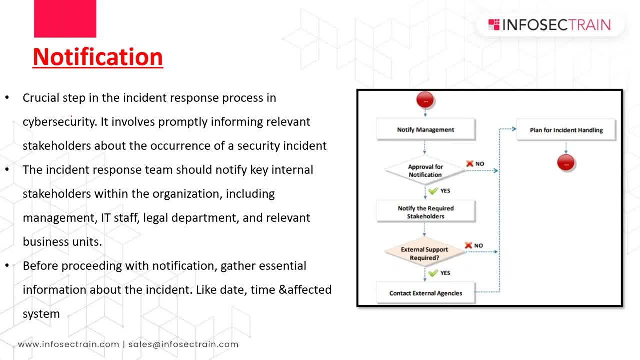 possible incident. right so, organization, an organization hit by a security incident, they need to notify the their appropriate or, you know, internal, external, you can say personal, so that they can minimize the, you know, incident. so this notification: they can basically save valuable assets from becoming vulnerable and help the individuals within the organization to play. 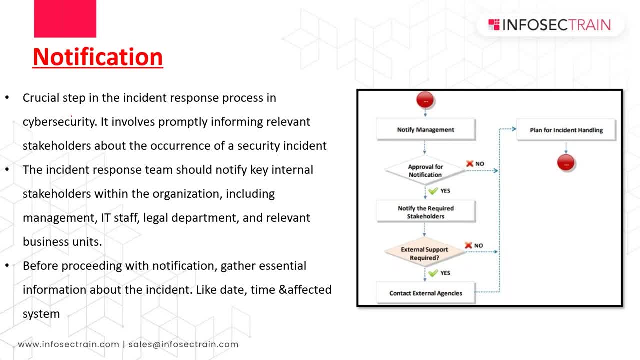 their- you know- respective rules. so in such a time, basically, cooperation can reduce the complexity and magnitude of resolving the security threat or incident. so effective communication is is crucial in incident response. to ensure, you know this, swift and coordinated actions. so communication will be helping to reduce the impact of an incident by enabling better 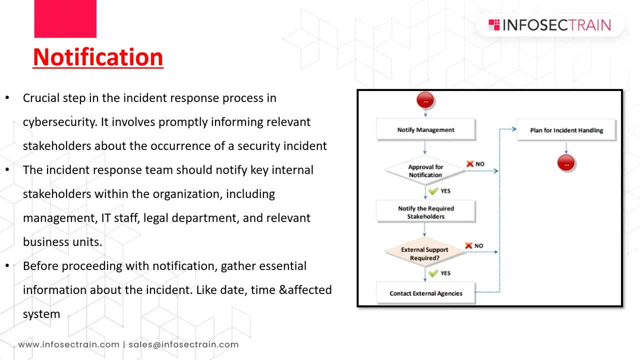 coordination among the stakeholders. incident handler: they must communicate, you know, the severity of the incident management and obtain their necessary approvals for performing the response procedures. okay, so communication. it can include various things, you know: sharing initial reports, assessment processes, detection methods, impacted resources, management strategies, all those things. and legal representative. they should be involved in discussion and legal actions may. 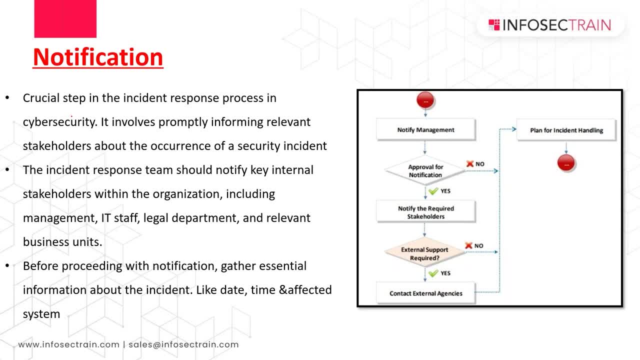 be pursued against the perpetrator right. so for that also, legal department or legal representative will also be included. so in incident handling response team when we talk about you know the legal let's are, they all um are included. so all employees and stakeholders. they should report security breach to the instant handling response. 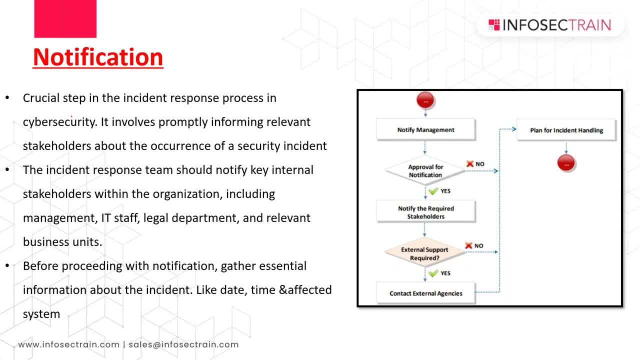 team instead of handling a response team. they lead discusses uh incident handling response team lead that discusses breaches with core team members and seeks for any external support if required. and after controlling the incident, the team will you know. they will disseminate the incident details and lesson loan will be there, the last one across the organization and to media also. okay, so 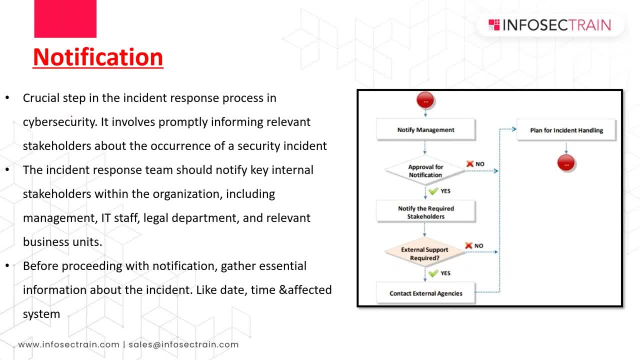 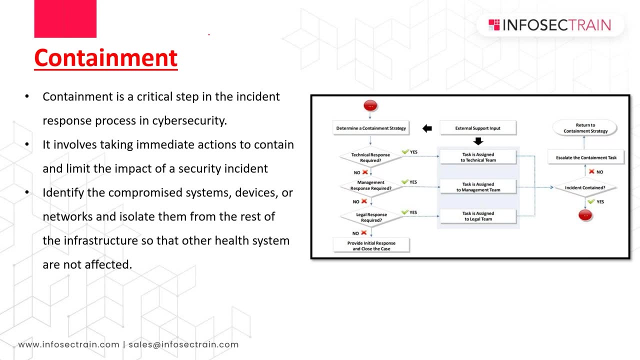 notification is required. side by side, i won't say: like to put your containment, uh, you know. after this i would say: continue. so when i say containment, what do you think containment is? for the same reason, if a malware got, in fact you know- inside a system, you can say: 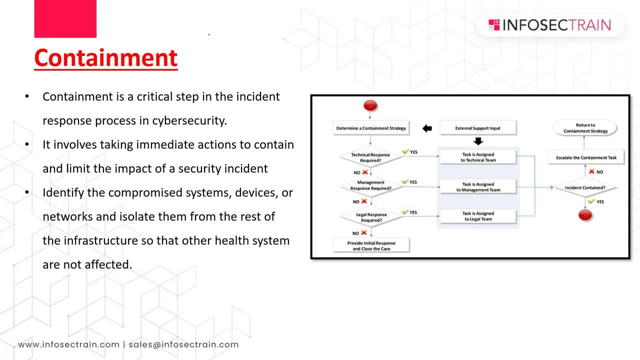 so obviously we'll put that system into a containment zone so that it won't spread out, right? we cut it down from the network, isn't it? so containment is a critical step in the incident response process in cyber security. it involves taking immediate actions to contain and 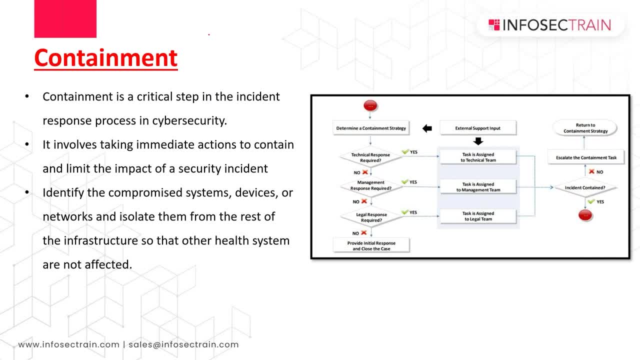 limit the impact of a security incident, identify the compromised systems, devices or networks and isolate them from the rest of the infrastructure so that other health systems are not affected. right, so i would say this goes side by side, because we cannot wait for the approvals of- uh you know, management or till the approval is there, because it can be. 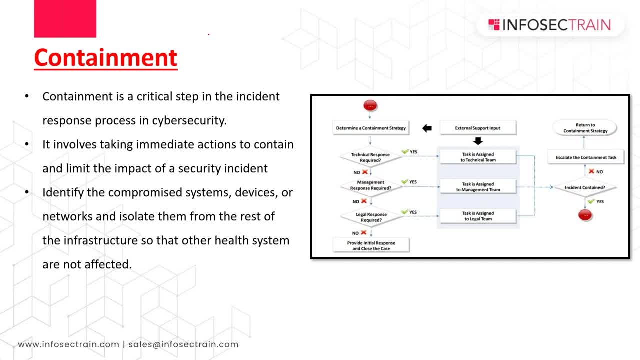 spread. so you can say, like containment goes hand in hand, sort of a way. because we don't, we want to cut down the impact as well. right, so this way? so process flow of containment starts with deciding the appropriate containment strategy for the particular type of incident. so then, depending 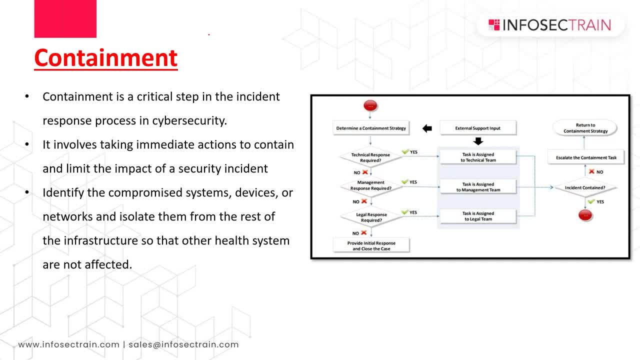 uh on the requirements of the technical response, management response and legal response to the incident. the task will be assigned to the technical team, management team or legal team respectively, in order to contain the incident. depending on the containment status, the containment task can be escalated back to the containment strategy stage so that they can 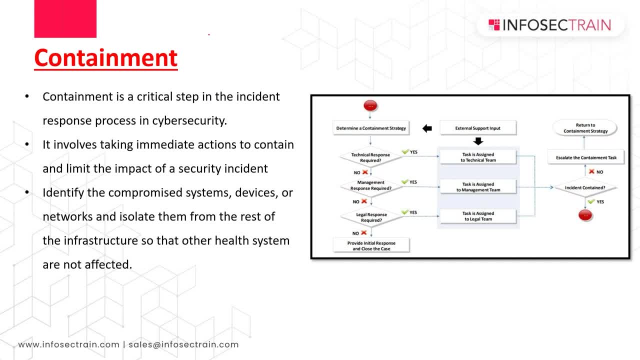 facilitate any modification to the strategy, if there is any, and after containment it goes for your own and the management team is required to complete the task so that they can execute the task. every day is gathering, okay. continuing is quite simple. over here you can see determine the continuous strategy, okay, like external support is required or not. so for 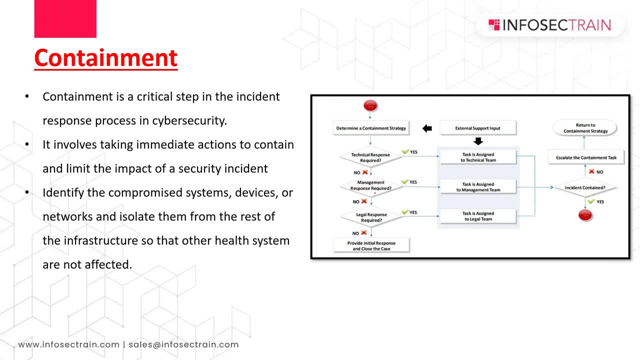 selecting a response required. yes, then task is sent to the technical team. if management is required, task is into management, legal to legal respectively. and uh, if everything is not required, then provide an initial response and close the case. if these teams are required, then incident is contained over. 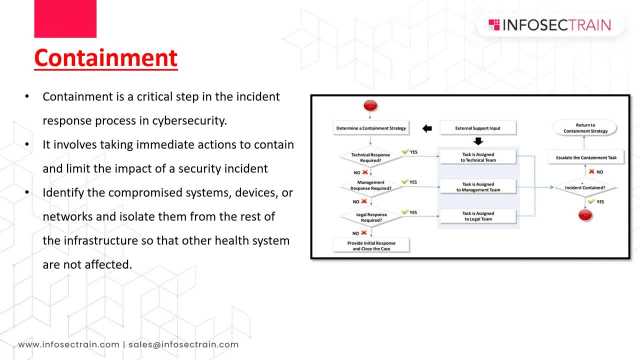 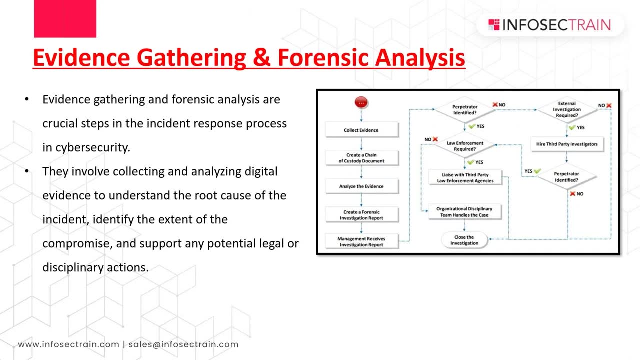 there then yeah, that's clear to containment task. containment strategy is done, that will be part of the containment. then from here it goes to your evidence gathering and forensic analysis, like i know. finding the root cause, that's what a forensic team does, or finding the perpetrator, as in the one who did this. 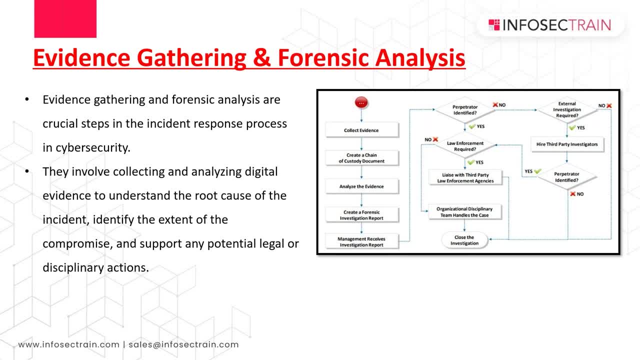 entire thing. so it focuses on removing the root cause of the incident, eliminating any malicious presence and ensuring that affected systems and networks are restored to a secure state. it may involve patching vulnerability or removing malware or restoring compromised data from team backups. right, okay, um, that will be for you can say: eradication, yeah, so evidence gathering and 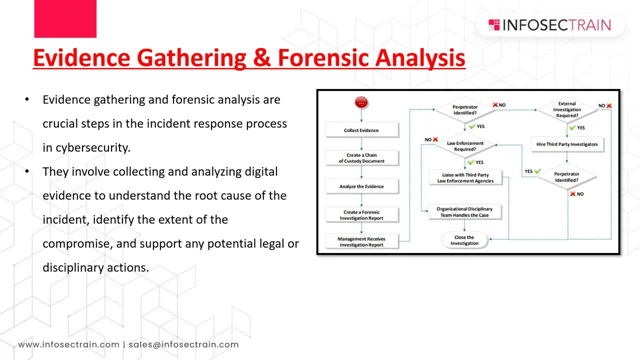 forensic analysis. as we said, like evidence gathering and forensic analysis, there are crucial steps in the incident response process in cyber security, like involving collecting, analyzing digital evidences to understand the root cause of the incident, identify the extent of the compromise and support any potential legal or any disciplinary actions are required. so, basically, over here, your incident handling. 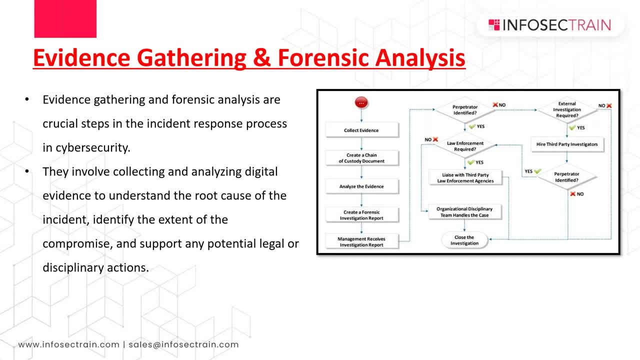 response team. they will collect crucial evidence and after this they'll go for the basically eradication which i was just talking about. so, incident handling response team, they will collect crucial evidences about the incident and then they will create a chain of custody document. there's a document which is created chain of custody. anyone knows what is chain of custody? 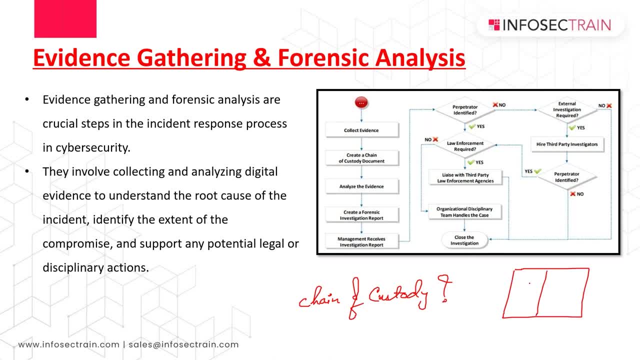 it's a chain of custody where you know that evidence- uh yeah, who all have handled that evidences will be entered or maintained in this particular chain of custody. the record will be maintained, at what time you handle, for what reason, and all those things in order to make sure, in case. 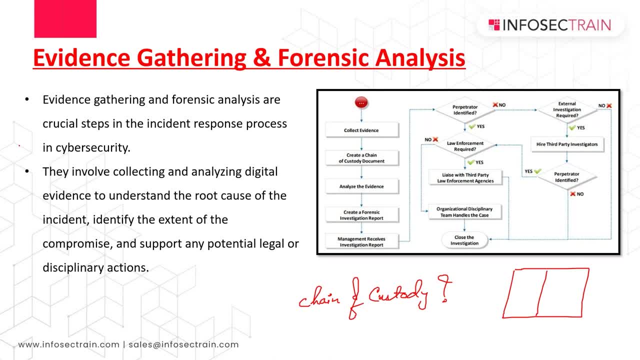 that if that evidence, when it, whenever it is, uh, submitted in front of court, you know if there is any changes found, this chain of custody can help you out, that you know where it got changed and who changed it. so for ensuring that chain of custody is there. okay, so chain of custody is that kind of a document. 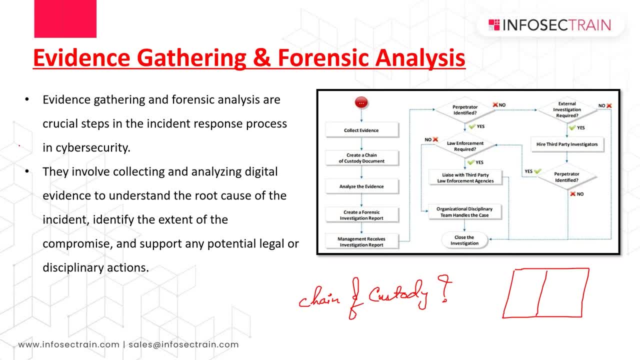 which holds entire information from the point when evidence was collected till the time it has been represented in front of court. who all handle that in evidence? at what time? at date, everything will be mentioned, that chain of custody, okay then. yeah, like what you just talked about, these are very unique, uh. 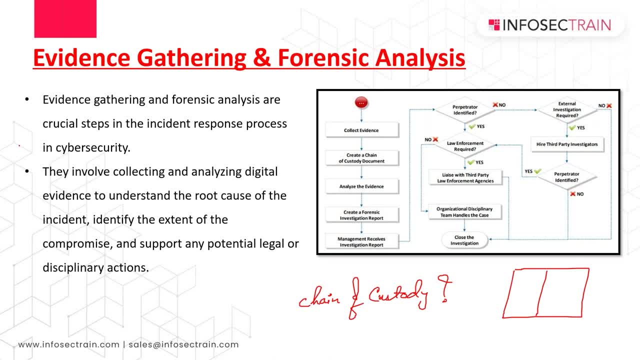 like you constantly give the record, no matter what. you don't answer this question. I, behind work, answer. now what I would say is: um, if you are a customer or if you are kind of a members like, not so what? what you need to do is you need to begin to work far beyond what you are first right and then after. 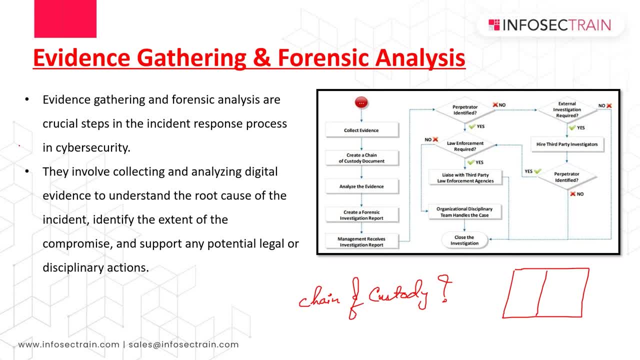 a lot of investigation. Gregory Bra sleeves, you understand now. I think krij is not sure about this way of working now, or that results very well. the problem is to management for further processing. so if the analysis can identify the perpetrator, then the management will decide whether they will legally prosecute the perpetrator or not. okay, 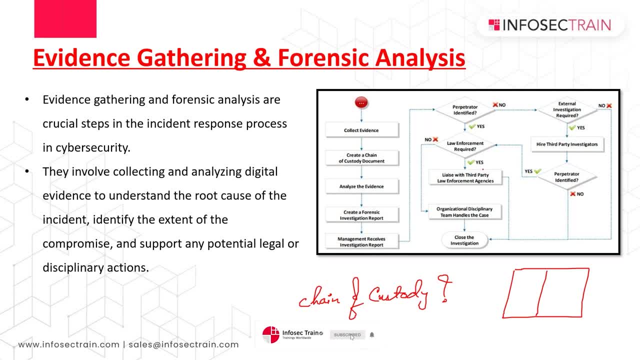 then the management will decide on their own whether they will handle this or not. so if the analysis can identify the perpetrator, management will decide whether they will legally prosecute the perpetrator or let the organization disciplinary team handle the case. if there is need of you know um need for law enforcement and management or a designated 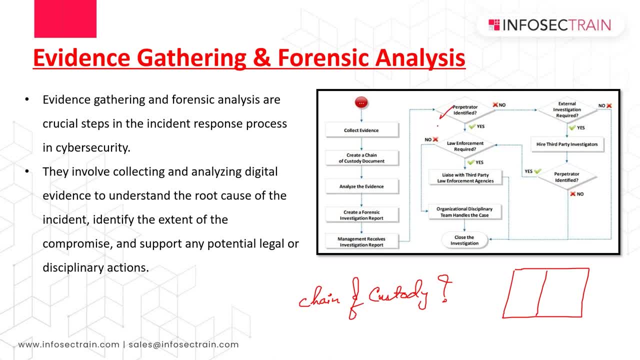 authority will contact a third party law enforcement agency. okay, then, they'll contact a third party law enforcement. okay, now the scene is like. if the investigation fails to identify the perpetrator or the detector, then management must decide whether to close the investigation or to pass it to an external. 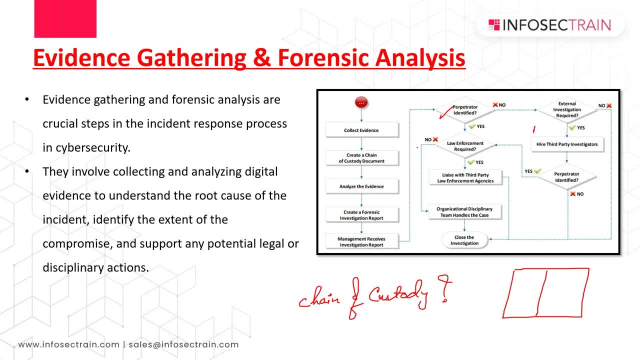 investigation. also, if they are able to identify the perpetrator, then that's fine, then it's everything is good. this normal process will be done. if operator was not identified by them, then management will be, like you know, giving approval, whether you want to go for the third party or 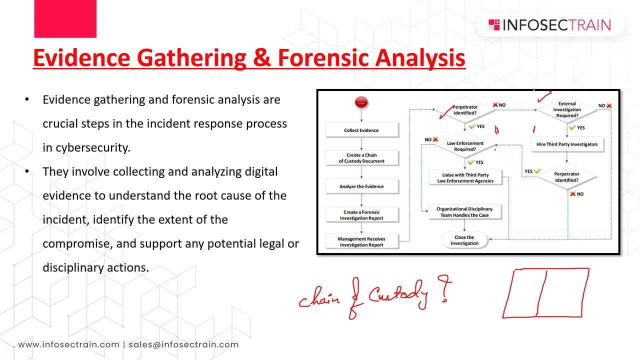 external investigating team or not. okay, so management must decide whether to close the investigation or to pass it to an external investigating or agency for further investigation if third party investigator can investigate the incident and if third party was able to identify the perpetrator right if they were able to identify. 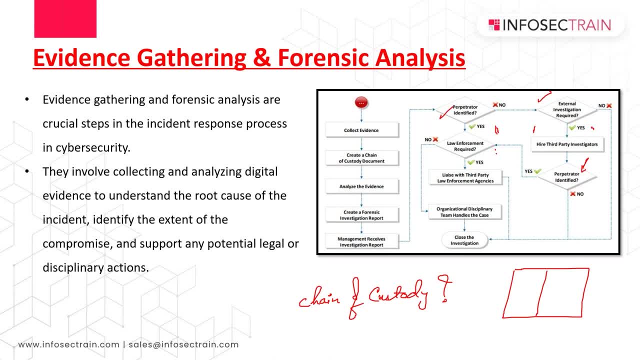 the perpetrator, then again same process. law enforcement required lies with third party law enforcement agencies and close investigation, right. so if law enforcement is not required, then again- which was happening in previously organization disciplinary team handles the case. if even third party is not able to handle or identify the perpetrator, then close the investigation. 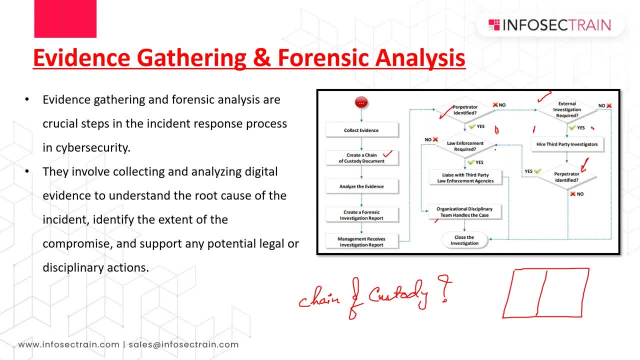 right away. okay, so you collect evidence, perform chain of custody, analyze the evidence, create a forensic investigation report. management receive the investigating report, the detailed one, and then they will decide like see if perpetrator is identified from within the organization against it, then if law enforcement is required, then fine. if law enforcement is required, then you go. uh, we check whether third party law enforcement. 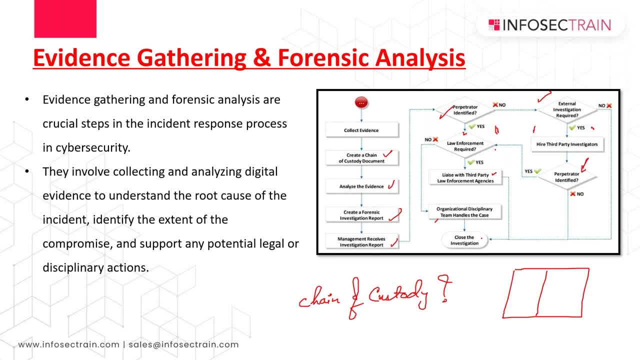 agency is there? if yes, then they will handle the thing and then close the investigation. if law enforcement is not required, organization disciplinary team will be handling the case and going with the punishment and close investigation. if perpetrator was not identified by ourselves, then we management will be looking. 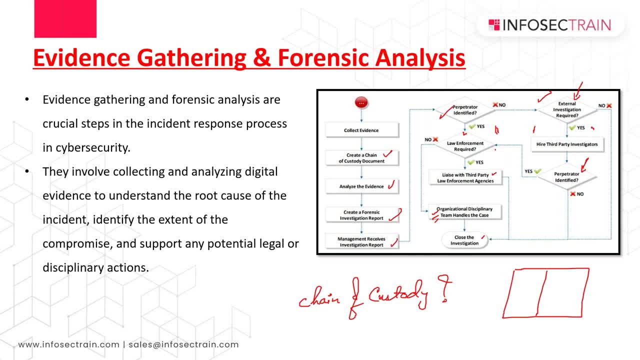 out for that, whether do we need to hire external investigation team or not. so if external investigation required, yes, then hired the third party investigator. okay, if not, close the case. if you are hiring third party investigator, if they are able to identify of or find the perpetrator, then again the same process if they are able to. if not, then again you have to go with the last. 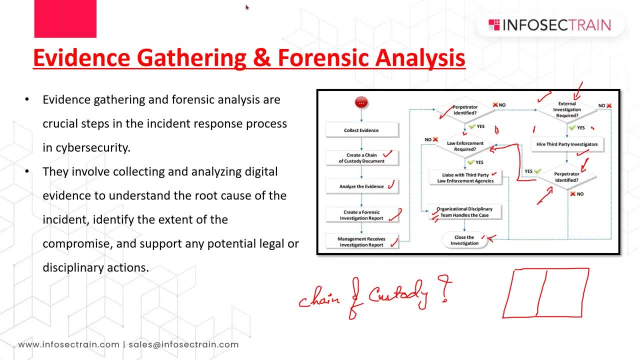 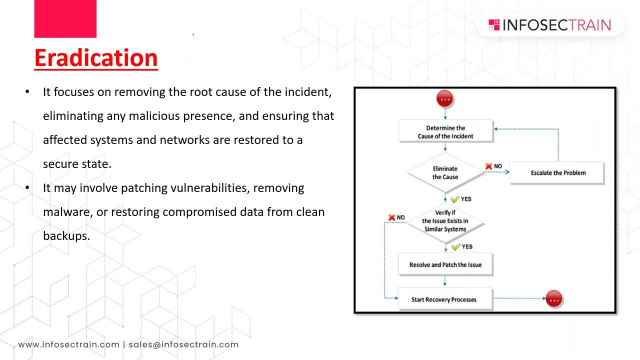 option, which is closer investigation. so this happens in your evidence gathering and forensic analysis, which brings you to the next one, which is eradication. eradication simply means what? as i mentioned, removal right. so it focused on removing the root cause of the incident, eliminating any malicious presence and ensure that affected systems and your network are restored to. 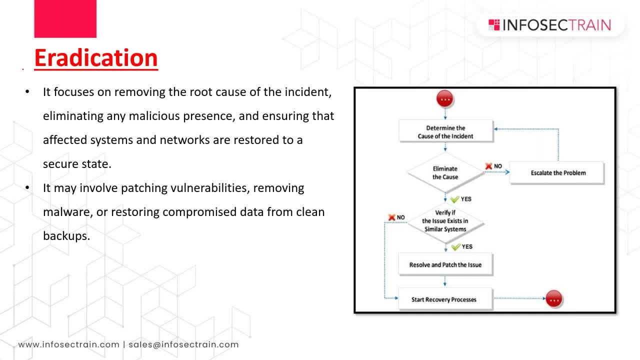 a secure state. so it may involve patching the vulnerabilities efforted everything at the same time moving malware or restoring the compromised data from clean backups. so after evidence gathering and forensic analysis, incident handling response team, they take action to eradicate the root cause of the incident. so team will be performing a vulnerability analysis to assess your network. 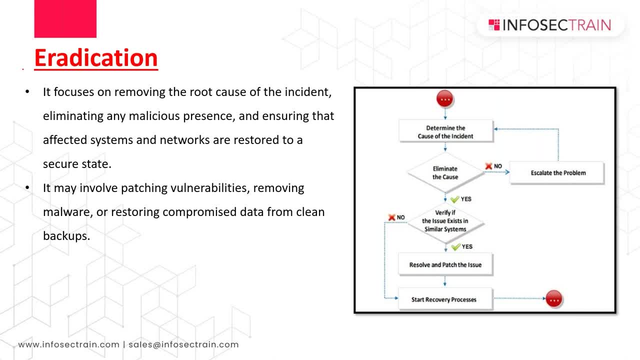 vulnerabilities and strengthen your network security. if the cause is still present, your team will try to eliminate it. otherwise, escalate the problem to the relevant departments. right, the team verifies if similar systems are affected and eliminate all the identified threats. so verify if this tissue or issue exists in similar system. yes, then it's all in pairs the issue from them as well. 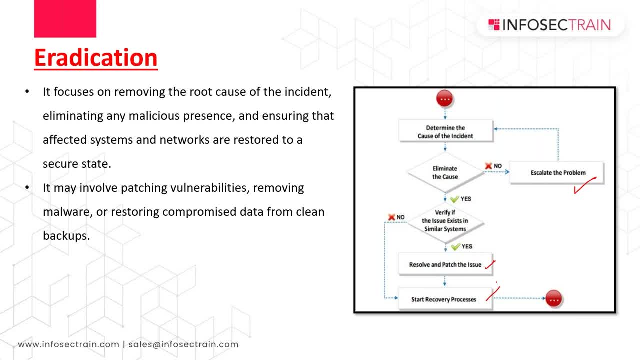 if not start the recovery process. so resolving the security post-it will be involving implementing protection tools, configuring network security devices, patching vulnerabilities. okay, so extreme cases, externally visible network component addresses. they may need to be changed, you know, to remove established attacking parts of it. and internal audits will be done of all the resources you know before initiating the recovery. 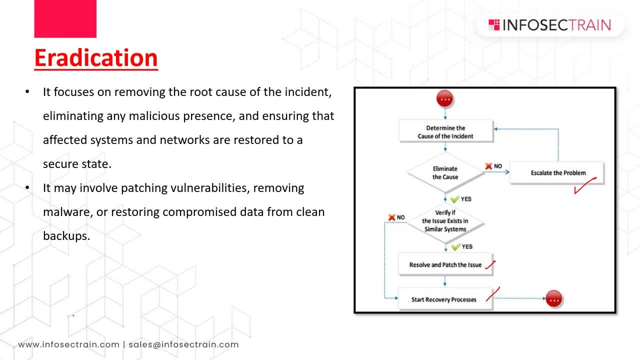 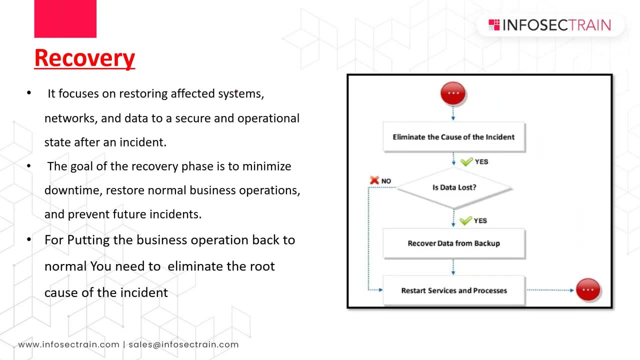 process to check various things into that. so these will be part of your eradication and then you go for the recovery at the end. recovery as in like using backups to you know, whatever the data has been lost to recover them back. so it focus on restoring affected system networks and data to 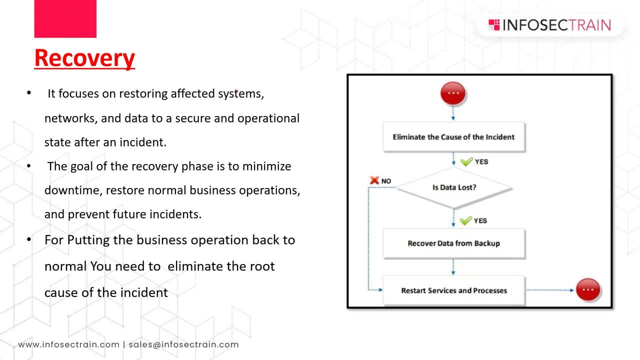 a secure and operational state after an incident. so the goal of the recovery phase is to minimize downtime right restore a normal business operations and prevent such future incidents. so for putting the business operation back to normal you need to eliminate the root cause of the incident first right. so 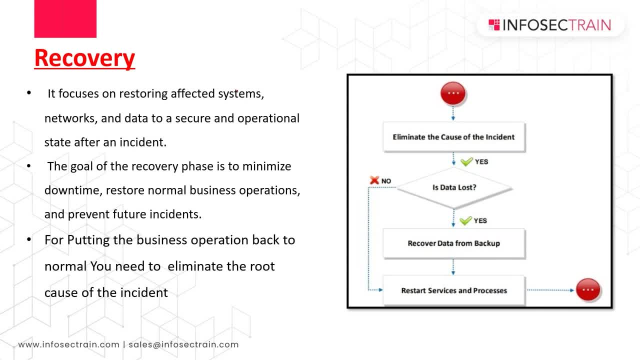 after eliminating the cause of the incident from all the system and resources. the incident handling response team they have to identify whether the data is lost. if the data is lost, then send handling response team has to recover the data from backups and restart the affected services and the processes in order to maintain the business continuity. I want to maintain the 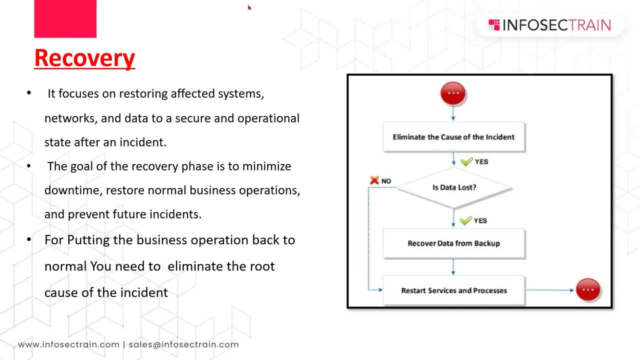 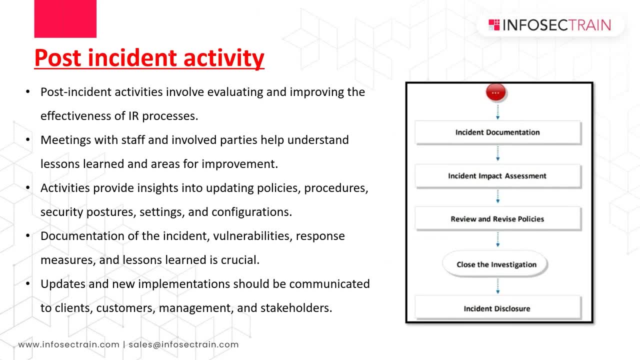 business continuity. okay, that brings to your post incident activity. the last one post incident activity involve evaluating and improving the effectiveness of incident response process. meeting with staff and involved parties help understand lesson learned- which I was talking about, the documentation part- and areas of improvement. so activities provide insights. 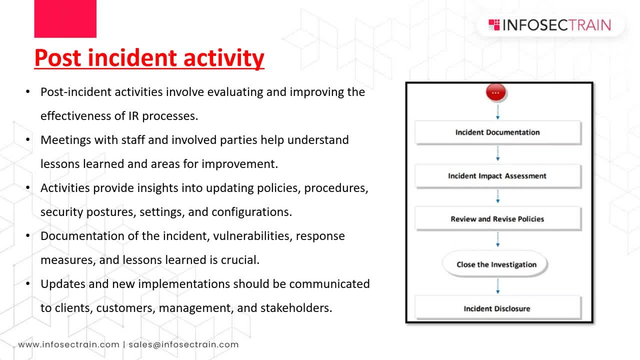 into updating policies, right uh procedures, security, posture settings, configuration. so documentation of the incident, the vulnerabilities, the response measures and lessons learned is crucial over here. so updates and new implementation. they should be communicated to clients, management and stakeholders post incident activity. they help in evaluating and improving the effectiveness of incident response processes by helping responders to assess any 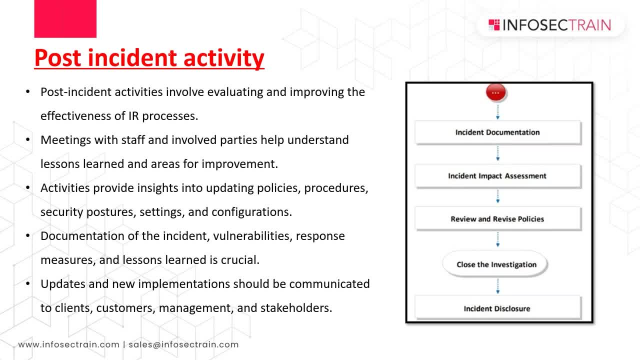 lags and security posture uh in security settings and configuration across their organization. they also help in suggesting, you know, measures and security products an organization can use to harden its security and optimize its policies. so to be sure organization they should conduct meetings with staff and other, you know, involved parties. 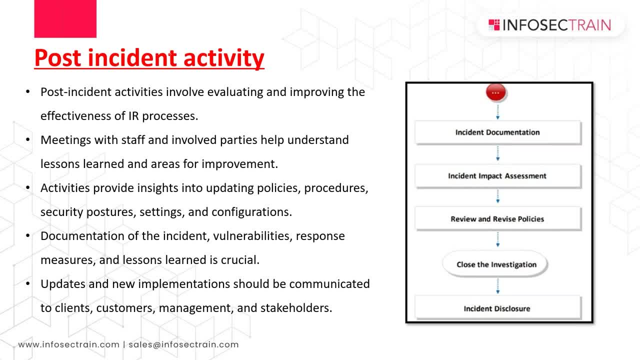 to understand all the lesson learned from the incident, and this will be helping him to improve in any areas in which it is you know currently Falls Behind. so these activities will help in evaluating and improving the effectiveness of response process by offering some insights into how to best update policies, procedures, security, 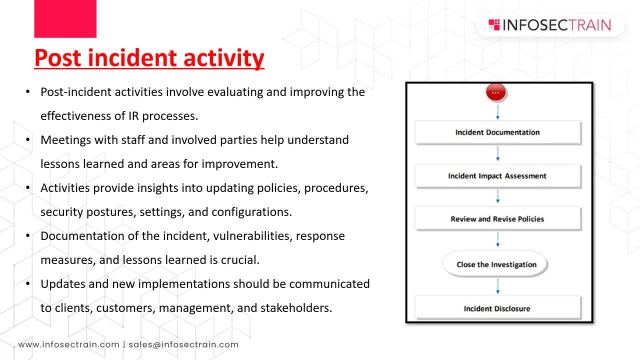 postures, settings and configurations across the organization to build a very robust network. okay, so, moreover, the- to learn from experience, you can say incident handling response team. they must have a document about the incident that reveals any details about the incident, of vulnerabilities exploited or response measures implemented or results any pitfall in the response processes. 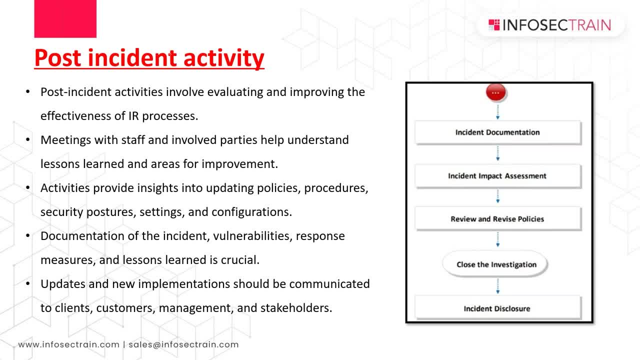 or drawbacks in communication management, everything, everything, basically. so these things have to be documented. so, accordingly, as you know, noted throughout this particular phases, incident handling response team: they should document every step of the instant response as well as the lesson they have implemented. so, instant handling response team: they must. 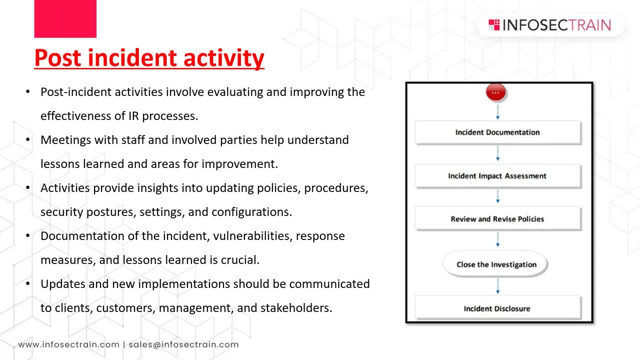 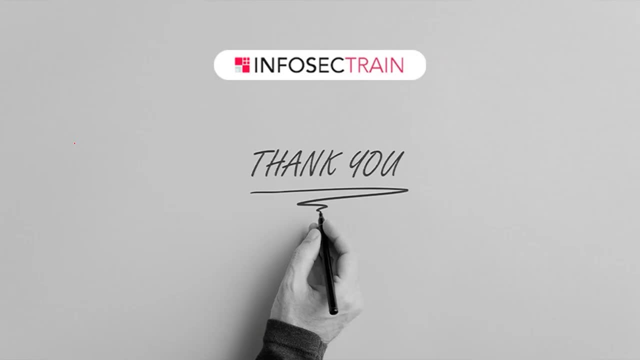 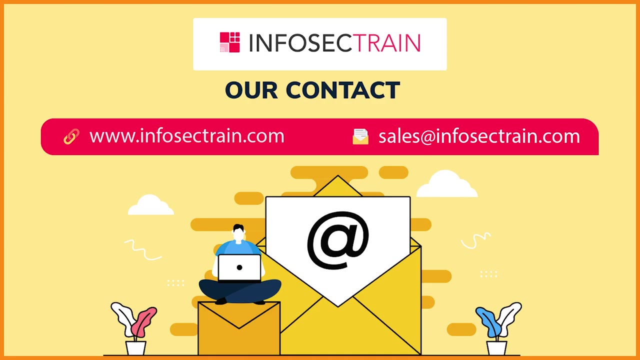 then communicate any updates and any new implementation to the clients, to the customers and the management and other stakeholders as well. so this is why it is important, okay, you.